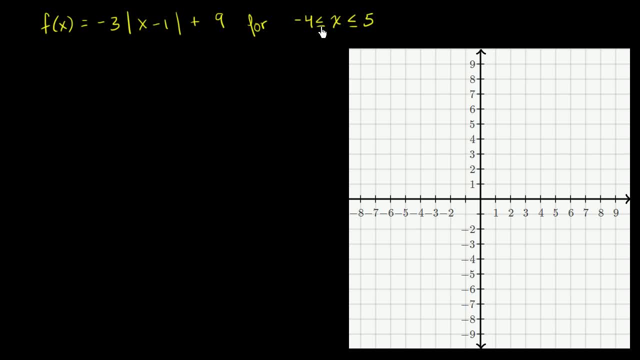 This is for x being or negative: 4 is less than or equal to x, which is less than or equal to 5.. And I encourage you to pause this video and try to graph this on your own, And clearly you could graph this by just trying out different x values. 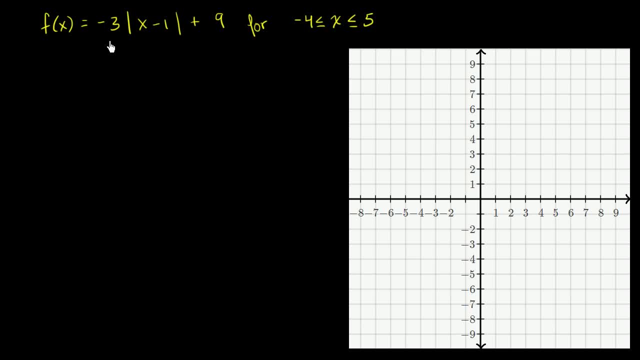 and plotting the corresponding x and f of x values. But really think about the structure of this expression And think about where does it hit a maximum or a minimum point And where would the vertex of it actually be? So let's look at this just holistically before we even try some points. 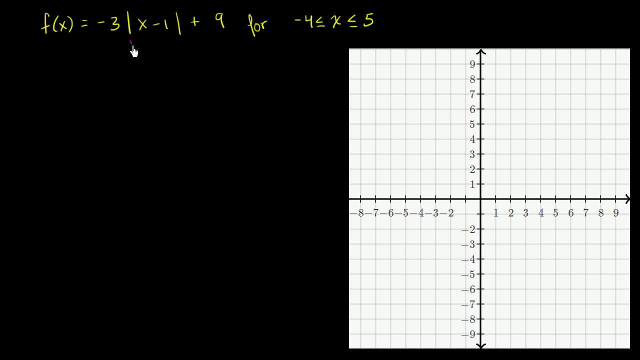 So we have an absolute value. This absolute value here is clearly going to always be non-negative. And then we're multiplying it. So we're multiplying it by, We're multiplying it by, We're multiplying it by a negative number. So this entire thing, you have a negative times, a non-negative. 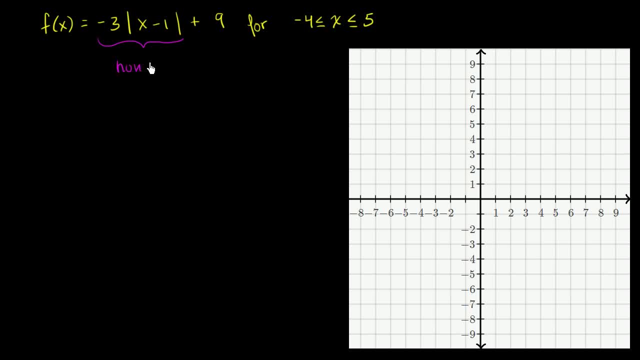 So this whole thing is always going to be non-positive. The reason why I say non-positive instead of negative is because it could be 0. So this whole part of the expression is either going to be 0 or it is going to be a negative number. 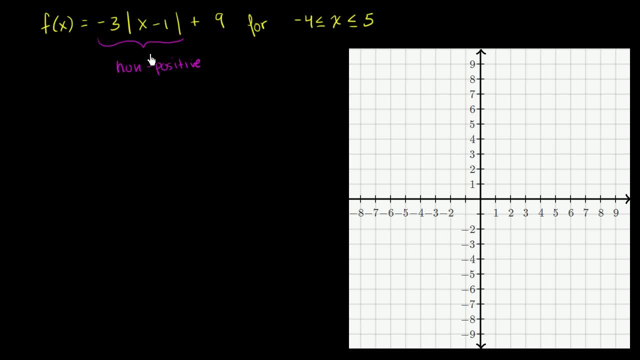 Now, if this is always non-positive, what is the maximum value of this function? Well, the maximum value happens when the absolute value is equal to 0. When the absolute value part of the expression is equal to 0, then this part is 0.. 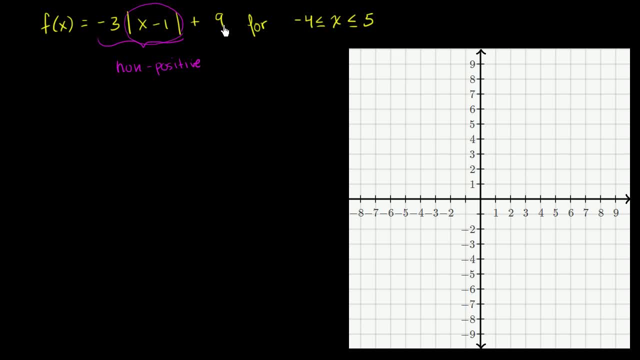 And the function hits its maximum value at f of x is equal to 9.. So when does the absolute value part of this expression equal 0?? Well, let's think about it. When does the absolute value of x minus 1 is going to be equal to 0?? 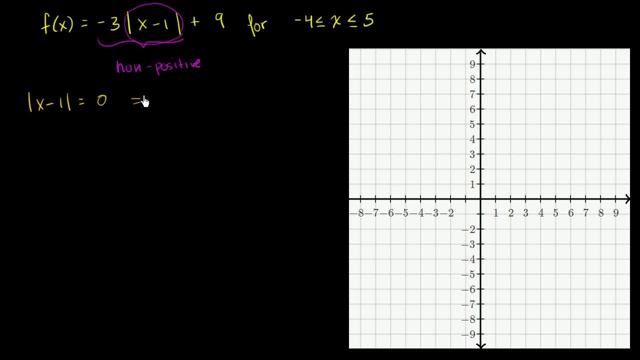 If x minus 1 is equal to 0, or if you add 1 to both sides, you get x is equal to 1.. So when x equals 1, we hit our maximum point. This thing becomes 0, which makes this whole thing equal to 0. 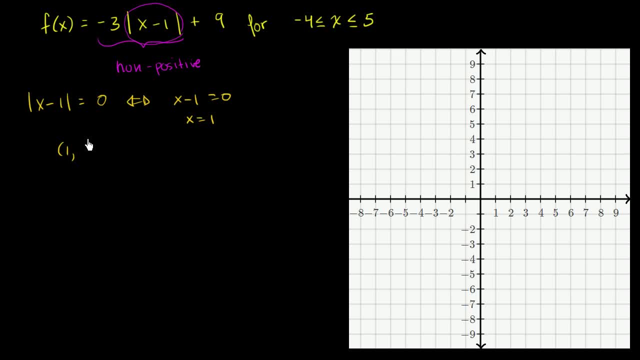 And so we get the point 1 comma 9.. So let's graph that point And actually let me do it. Let me do it in a column. This is the color that's easier to see on a white background. 1 comma 9 is the maximum point right over here. 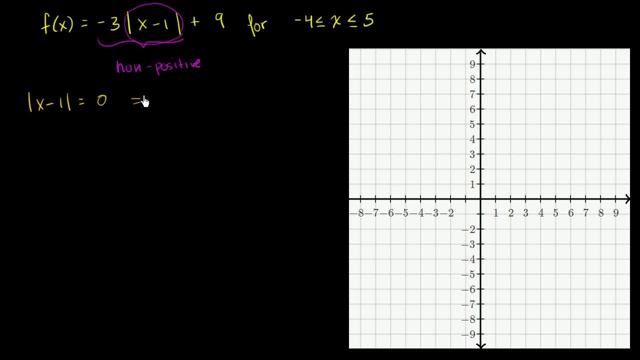 If x minus 1 is equal to 0, or if you add 1 to both sides, you get x is equal to 1.. So when x equals 1, we hit our maximum point. This thing becomes 0, which makes this whole thing equal to 0. 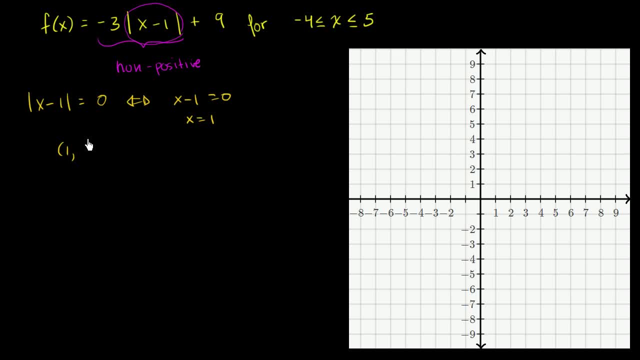 And so we get the point 1 comma 9.. So let's graph that point And actually let me do it. Let me do it in a column. This is the color that's easier to see on a white background. 1 comma 9 is the maximum point right over here. 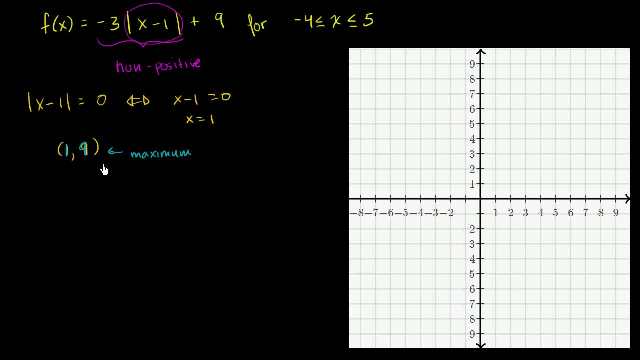 And in the case you could also view this as the vertex of this absolute value function. So 1 comma 9 is that point right over there, And so we can already guess the general shape of this. An absolute value function either looks something like that: 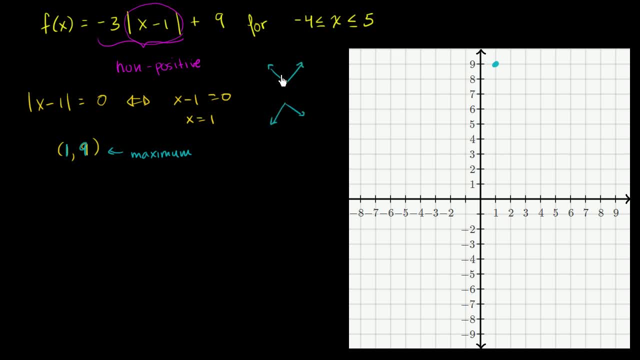 or it looks something like that. It would look like this: If the coefficient right over here- or I guess I shouldn't call it a coefficient- the thing multiplying the absolute value- was positive, then it would be upward opening, like that. But since it is negative, it is going to be downward opening. 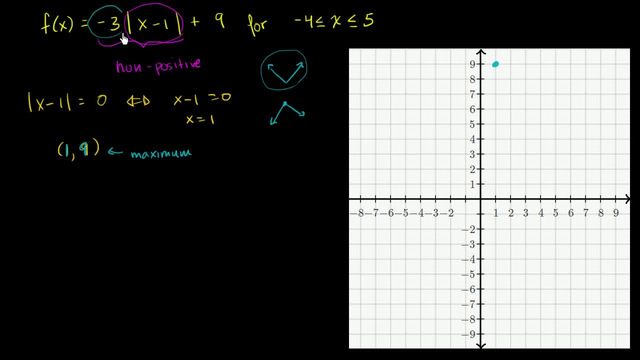 We hit a maximum point at the vertex, in this case we're just talking about, for the reasons we just discussed. But then what happens there? What happens to the right of that vertex And what happens to the left of this vertex? Well, we don't have to do it this way. 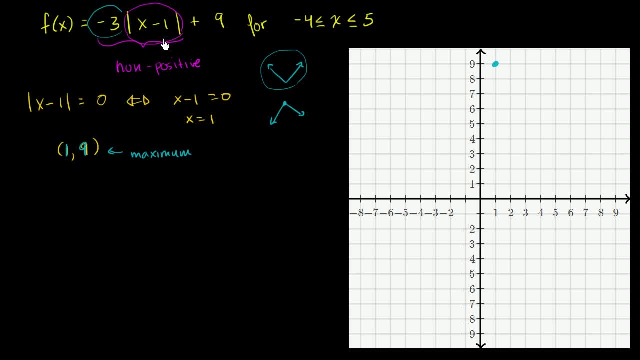 Once again, You could just try out points if you like, But I like to really analyze what's going on here. So let's break up this function definition into two pieces. So let's say that f of x is equal to. We're going to break it up into two pieces, one piece. 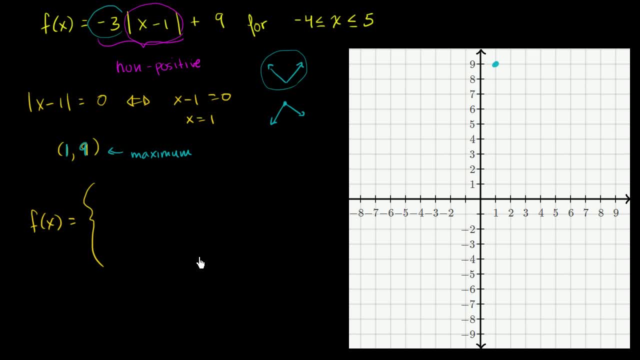 to the right of the vertex and one piece to the left of the vertex. So to the right of the vertex that's going to be: 1 is less than or equal to x, which is less than or equal to 5.. And to the left of the vertex, so this: 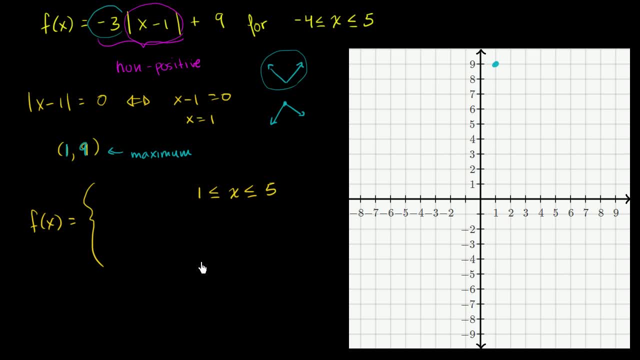 is to the right of the vertex, to the left of the vertex. that's going to be- let me do this in a different color- that's going to be negative. 4 is less than or equal to x, And I'll say less than 1.. 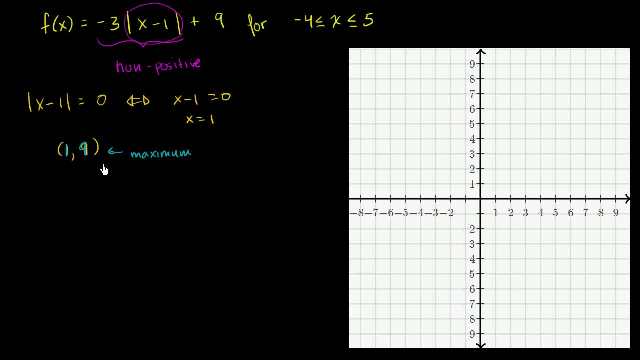 And in the case you could also view this as the vertex of this absolute value function. So 1 comma 9 is that point right over there, And so we can already guess the general shape of this. An absolute value function either looks something like that: 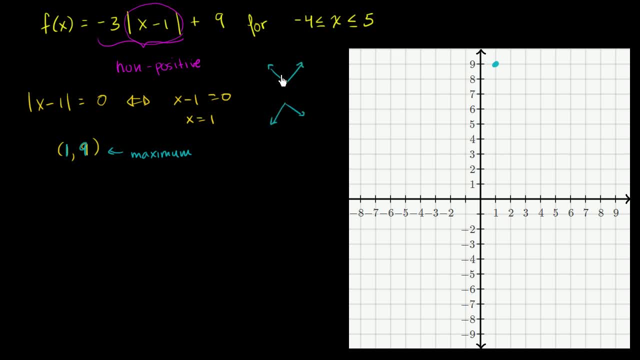 or it looks something like that. It would look like this: If the coefficient right over here- or I guess I shouldn't call it a coefficient- the thing multiplying the absolute value- was positive, then it would be upward opening, like that. But since it is negative, it is going to be downward opening. 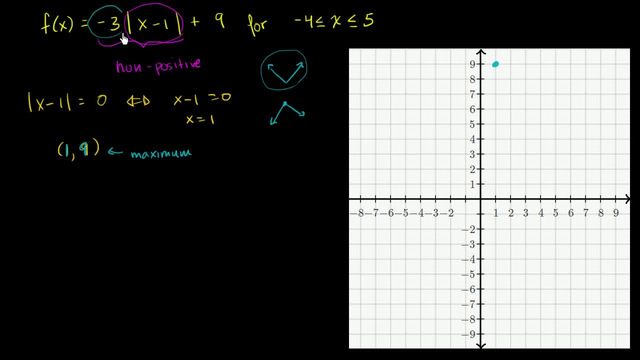 We hit a maximum point at the vertex, in this case we're just talking about, for the reasons we just discussed. But then what happens there? What happens to the right of that vertex And what happens to the left of this vertex? Well, we don't have to do it this way. 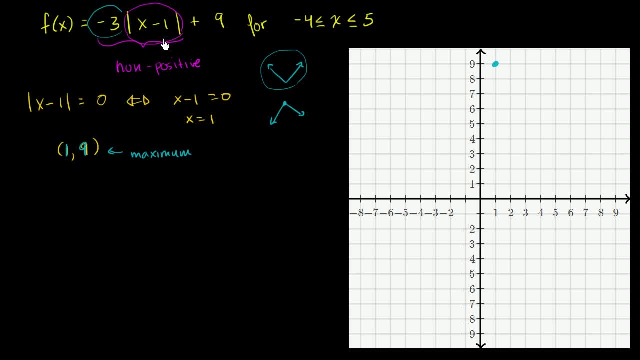 Once again, You could just try out points if you like, But I like to really analyze what's going on here. So let's break up this function definition into two pieces. So let's say that f of x is equal to. We're going to break it up into two pieces, one piece. 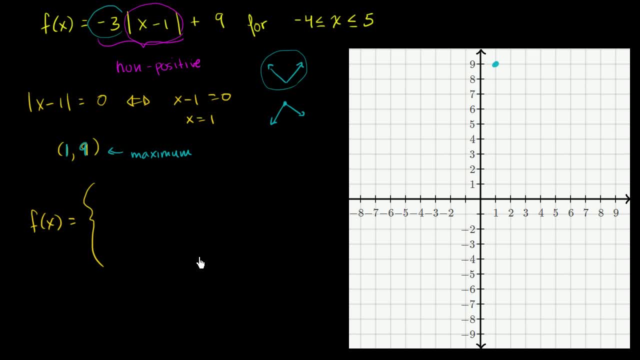 to the right of the vertex and one piece to the left of the vertex. So to the right of the vertex that's going to be: 1 is less than or equal to x, which is less than or equal to 5.. And to the left of the vertex, so this: 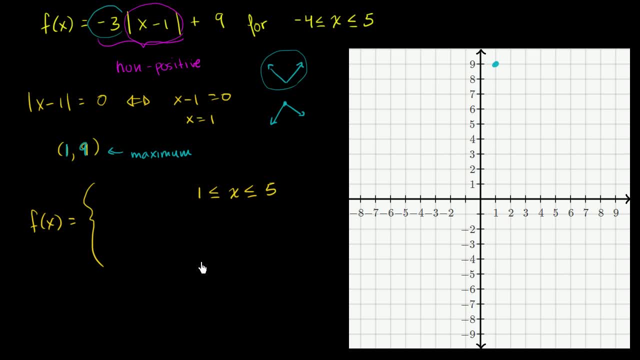 is to the right of the vertex, to the left of the vertex. that's going to be- let me do this in a different color- that's going to be negative. 4 is less than or equal to x, And I'll say less than 1.. 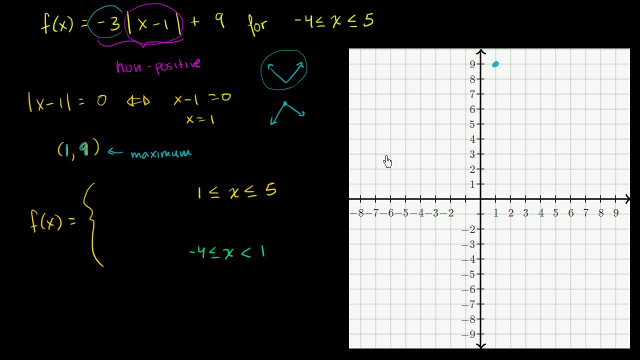 So just to be clear, our whole domain was between negative 4 and 5.. Between negative 4 and 5 was our entire domain. Now I'm breaking it up to the right of the vertex and the left of the vertex. So this right over here is to the right of the vertex. 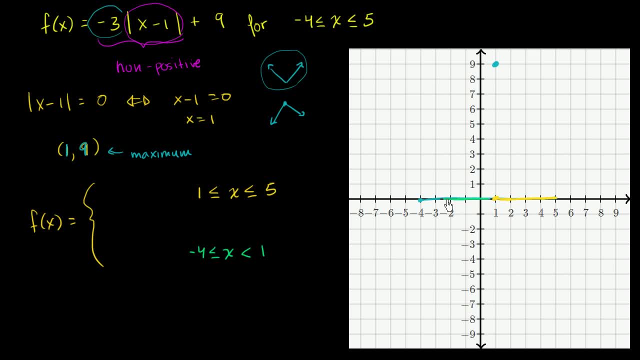 and this right over here is to the left of the vertex, So to the right of the vertex, for x being greater than or equal to 1, this absolute value, or one way to think about it, when x is greater than or equal. 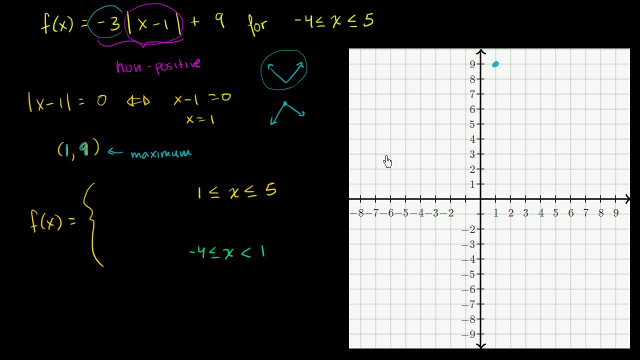 So just to be clear, our whole domain was between negative 4 and 5.. Between negative 4 and 5 was our entire domain. Now I'm breaking it up to the right of the vertex and the left of the vertex. So this right over here is to the right of the vertex. 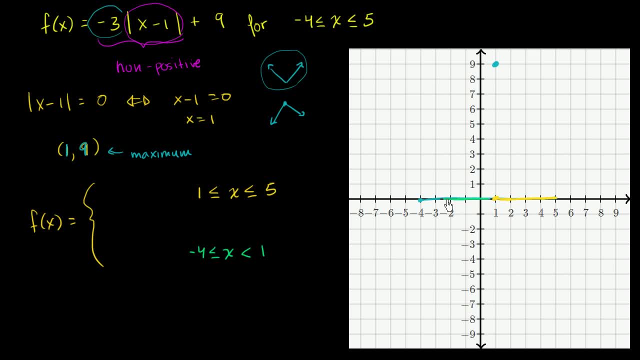 and this right over here is to the left of the vertex, So to the right of the vertex, for x being greater than or equal to 1, this absolute value, or one way to think about it, when x is greater than or equal. 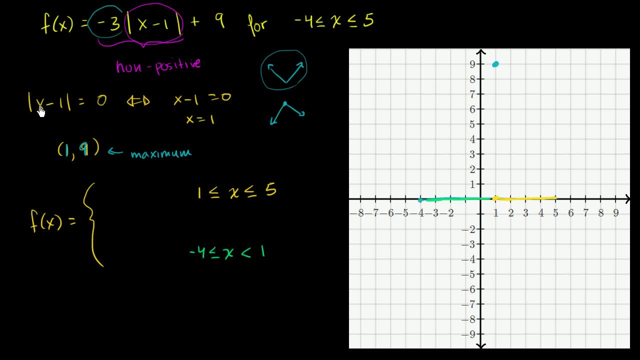 to 1, x minus 1 is going to be positive, And the absolute value of a positive thing is just going to be that same value. So for x is greater than or equal to 1, our function is going to be negative 4.. 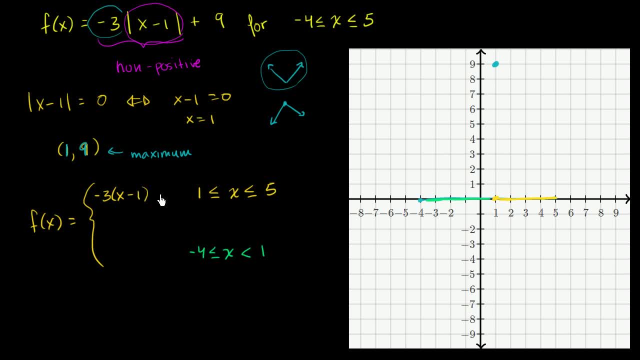 Negative 3 times x minus 1 plus 9.. Or if you wanted to distribute the negative 3, this would be the same thing. Actually, let me write it over here so that we can write the simplified version. So it would be. let me give myself some space. 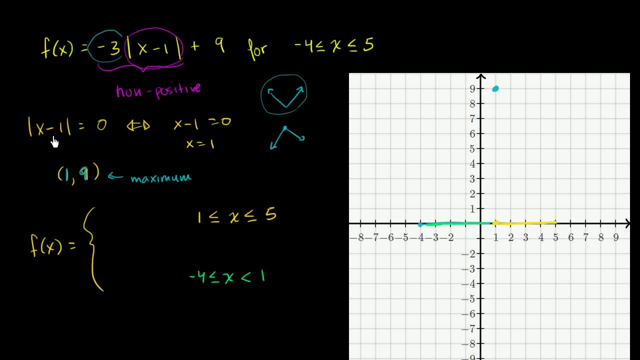 So for x is greater than or equal to 1, we don't have to think about the absolute value. So it would be negative 3 times x minus 1 plus 9, which is negative 3x Plus 3x. 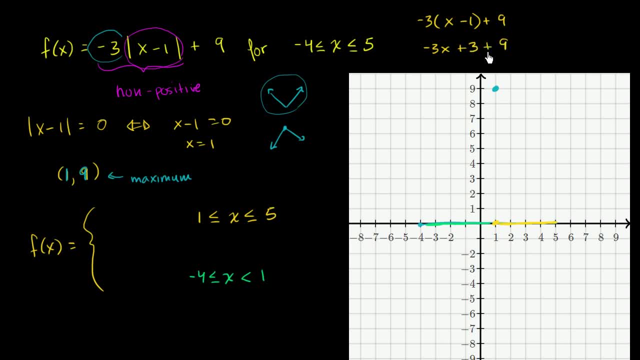 3 plus 9, or negative 3x plus 12.. So it's going to be negative 3x plus 12 when x is greater than or equal to 1.. And the really interesting thing is here is the slope here is negative. 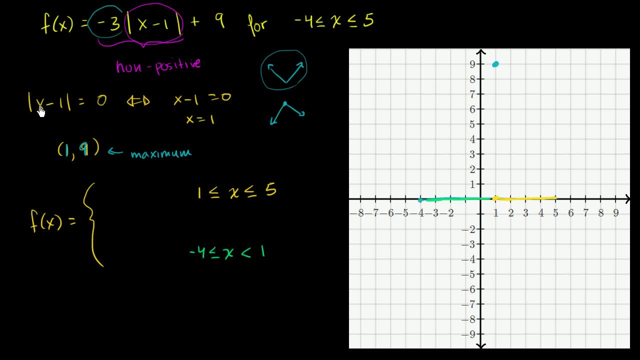 to 1, x minus 1 is going to be positive, And the absolute value of a positive thing is just going to be that same value. So for x is greater than or equal to 1, our function is going to be negative 4.. 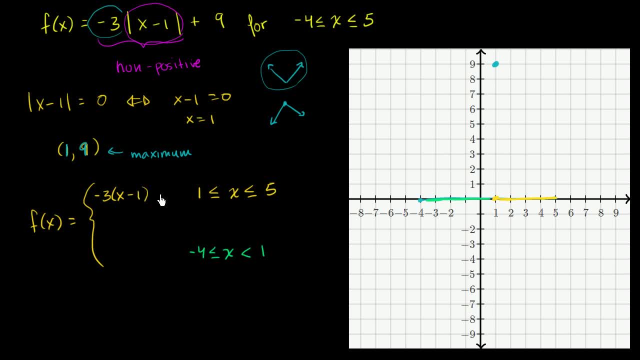 Negative 3 times x minus 1 plus 9.. Or if you wanted to distribute the negative 3, this would be the same thing. Actually, let me write it over here so that we can write the simplified version. So it would be. let me give myself some space. 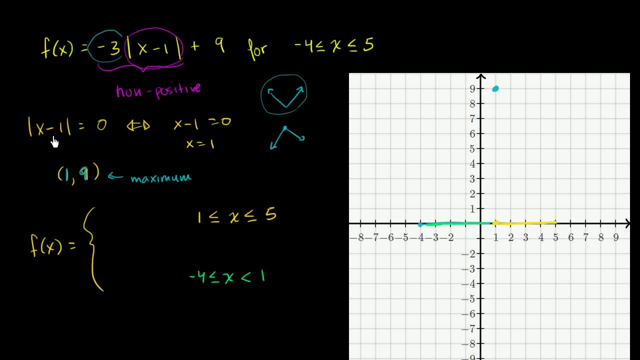 So for x is greater than or equal to 1, we don't have to think about the absolute value. So it would be negative 3 times x minus 1 plus 9, which is negative 3x Plus 3x. 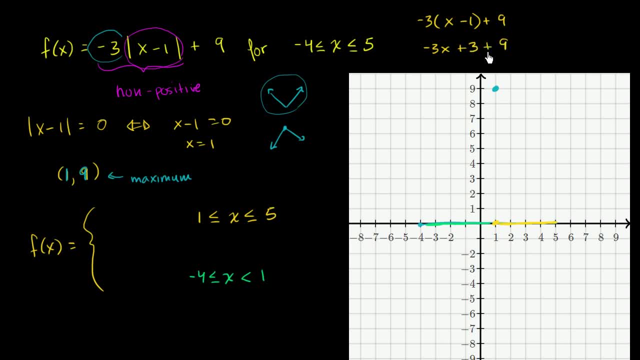 3 plus 9, or negative 3x plus 12.. So it's going to be negative 3x plus 12 when x is greater than or equal to 1.. And the really interesting thing is here is the slope here is negative. 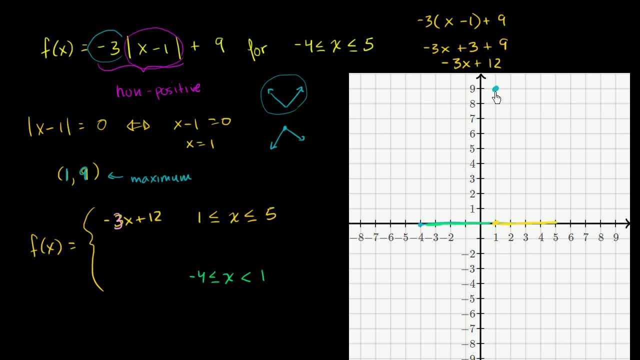 We have a slope of negative 3.. So, starting from this point, if we have a slope of negative 3, that means every time we move 1 in the x direction, we're going to decrease by 3 in the y direction. 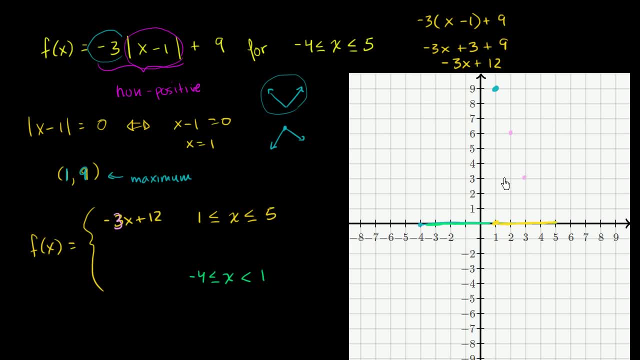 Increase by x, Decrease. Decrease by y, by 3.. So it's a slope of negative 3.. So it will look like that, And let me actually do it in purple so that you can actually see it. That's not purple. 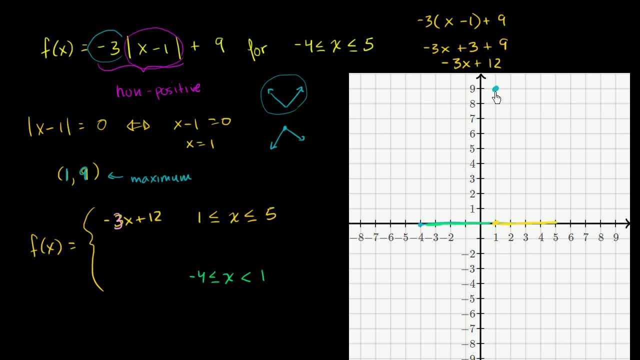 We have a slope of negative 3.. So, starting from this point, if we have a slope of negative 3, that means every time we move 1 in the x direction, we're going to decrease by 3 in the y direction. 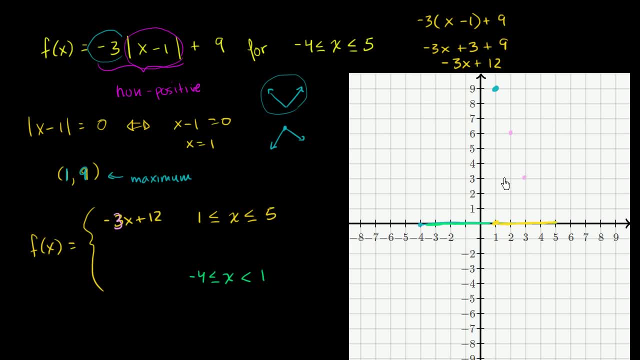 Increase by x, Decrease. Decrease by y, by 3.. So it's a slope of negative 3.. So it will look like that, And let me actually do it in purple so that you can actually see it. That's not purple. 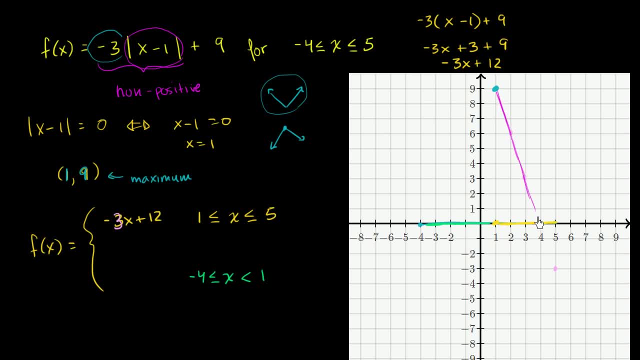 There you go. That's purple, All right. So it would look like that, And actually let me just make it clear This is what I'm talking about right over here. That piece of the function is going to look like that. 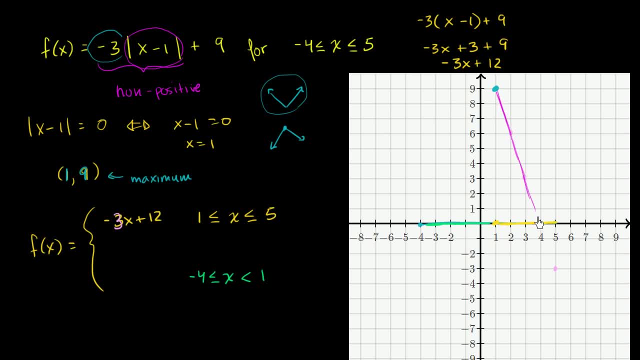 There you go. That's purple, All right. So it would look like that, And actually let me just make it clear This is what I'm talking about right over here. That piece of the function is going to look like that. 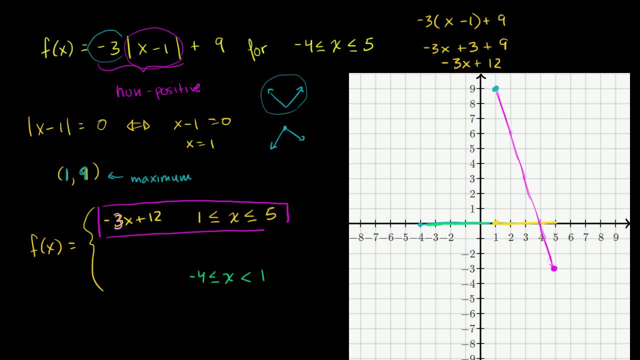 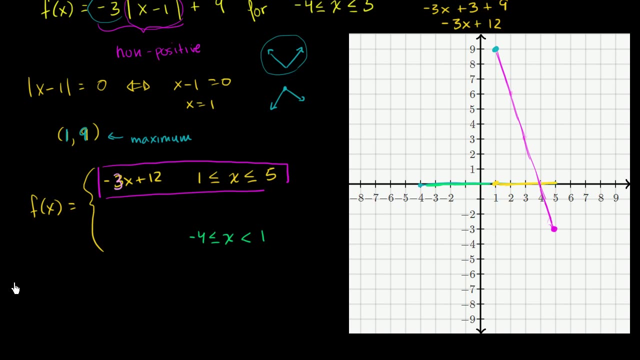 Now what about when x is less than 1?? Well, when x is less than 1, x minus 1 is going to be negative, And so the absolute value is going to be the negative of that actual function. So when x is less than 1, the absolute value of x minus 1. 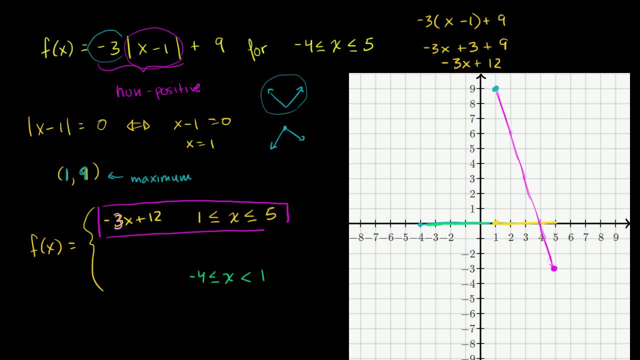 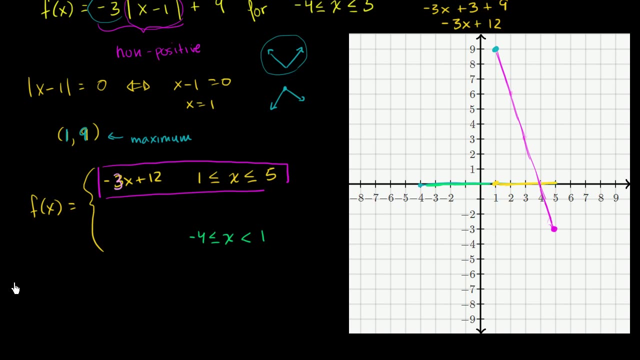 Now what about when x is less than 1?? Well, when x is less than 1, x minus 1 is going to be negative, And so the absolute value is going to be the negative of that actual function. So when x is less than 1, the absolute value of x minus 1. 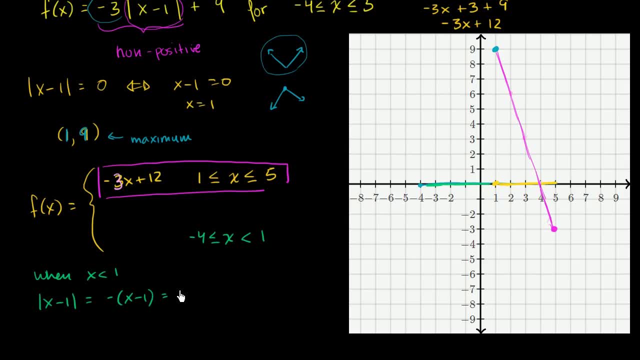 is equal to the negative of x minus 1, which is the same thing as 1 minus x. So our function is going to be negative. So our function is going to be negative. So our function is going to be negative 3 times 1 minus x. 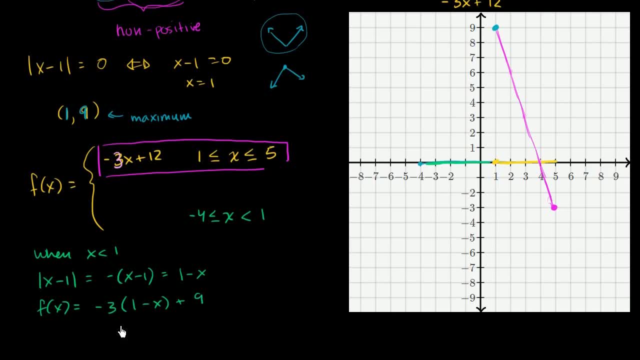 plus 9,, which is the same thing as. let's see, if you distribute the negative 3, it's negative 3 plus 3x plus 9, which is equal to 3x plus 6.. So the important thing is 3x plus 6.. 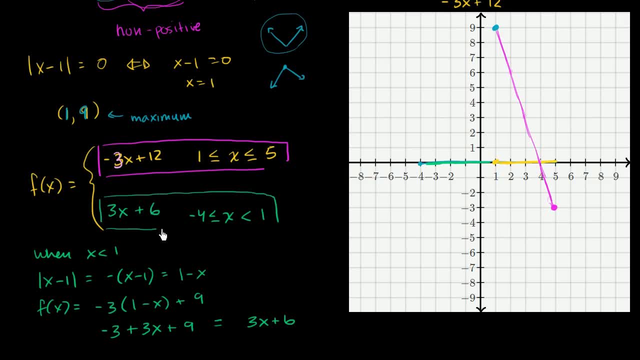 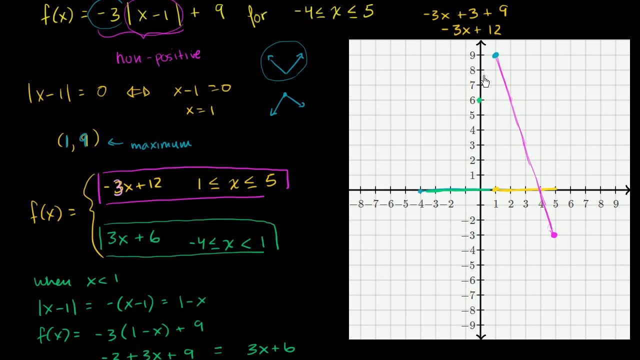 The important thing to realize here is that our slope is positive 3. Our slope is positive 3. And you could even say that we have a y-intercept here at 6.. So it would be this point right over here, And the line would look like this: 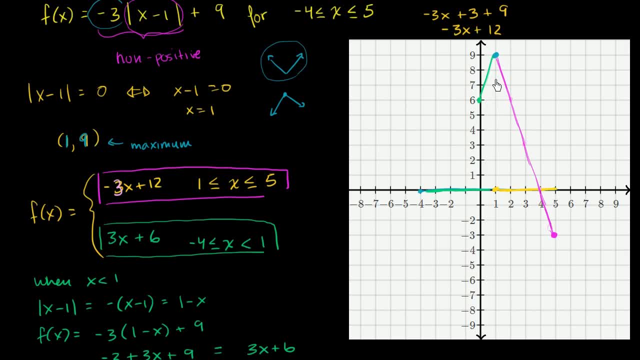 When your slope is positive 3,, you increase x by 1, you increase y by 3.. Increase x by 1,, increase y by 3.. Or another way of thinking about it: if you decrease x by 1,, then you decrease y by 3.. 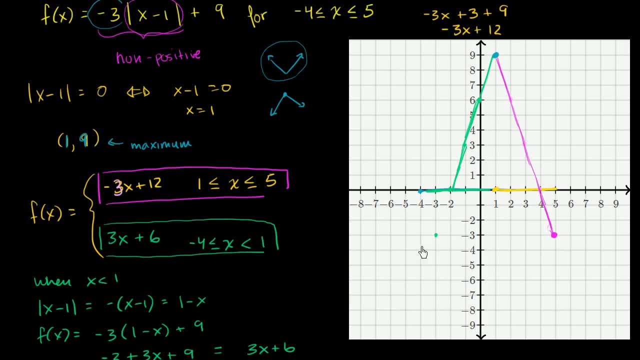 Decrease x by 1,. decrease y by 3.. Decrease x by 1,. decrease y by 3.. So it would look like that, And we are done. We have graphed this absolute value equation. Now the whole reason why I did this. 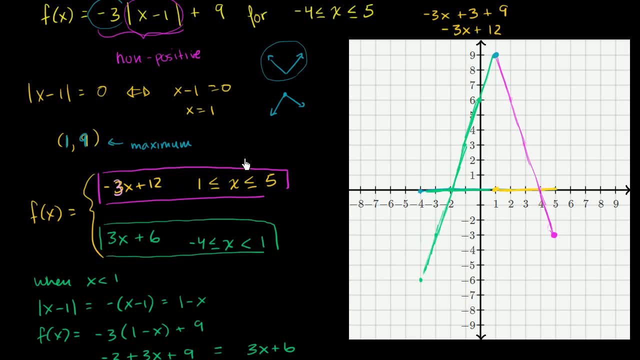 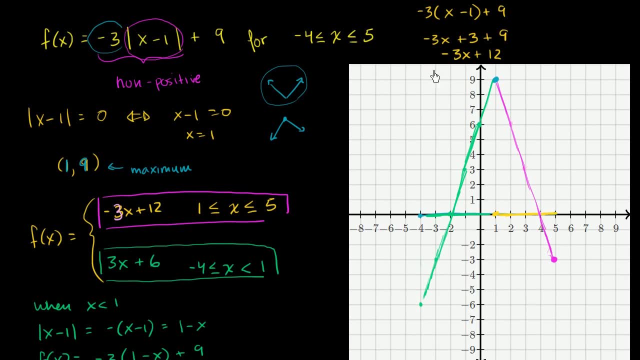 is so that we learn it a little bit deeper. But there would have been a faster way of doing this. You could have just said: hey, this is going to hit a maximum point when x is equal to 1, because this non-positive thing is going to hit 0.. 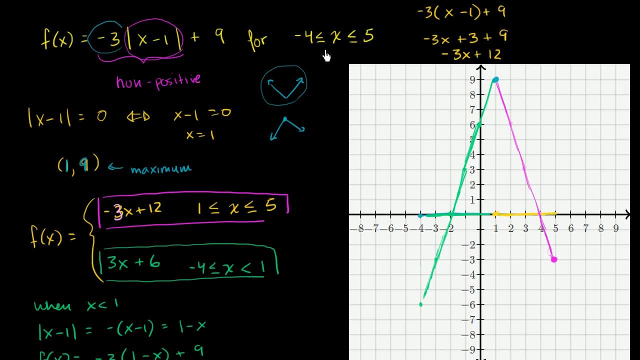 So you could have said 1 comma 9 is the vertex, And then you could have just tried out the two endpoints, knowing that between the endpoints and the vertex you're essentially just dealing with the lines. You could have just evaluated f of negative 4,. 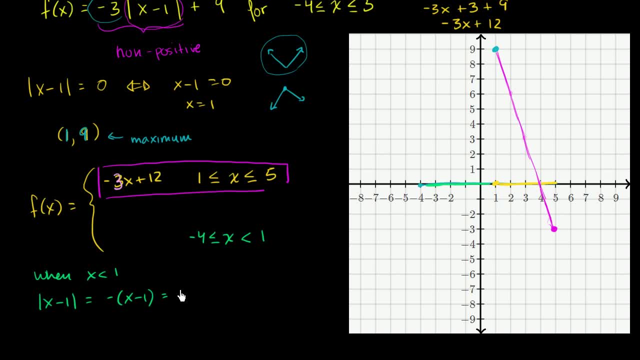 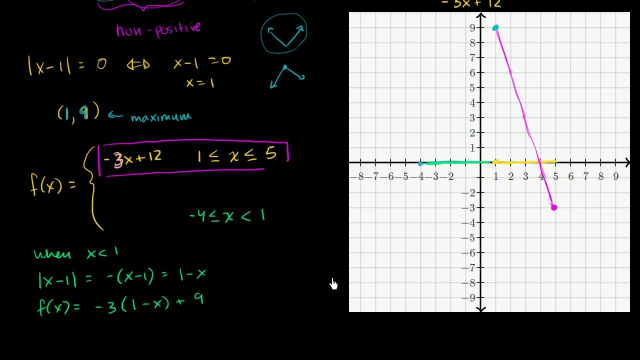 is equal to the negative of x minus 1,, which is the same thing as 1 minus x. So our function is going to be negative. So our function is going to be negative 3 times 1 minus x plus 9,, which is the same thing as. let's see: 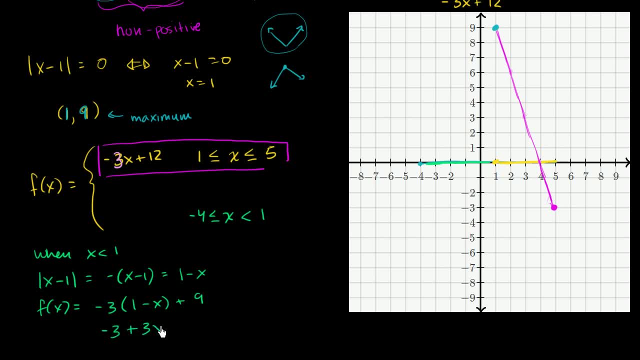 if you distribute the negative 3, it's negative 3 plus 3x plus 9, which is equal to 3x plus 6.. So the important thing is 3x plus 6.. The important thing to realize here is that our slope is positive 3.. 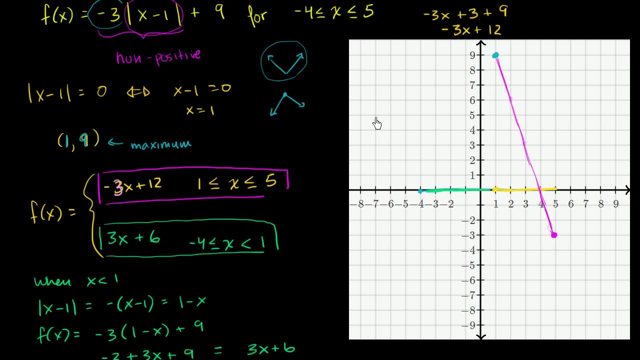 Our slope is positive 3.. And you could even say that we have a slope, We have a y-intercept here at 6.. So it would be at this point, right over here, And the line would look like this: When your slope is positive 3,, you increase x by 1,. 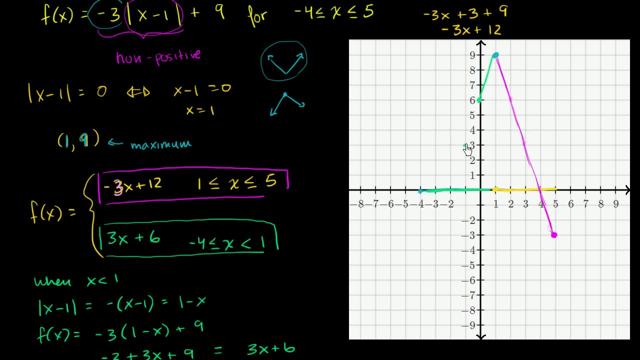 you increase y by 3.. Increase x by 1,, increase y by 3.. Or another way of thinking about it: if you decrease x by 1,, then you decrease y by 3.. Decrease x by 1,, decrease y by 3.. 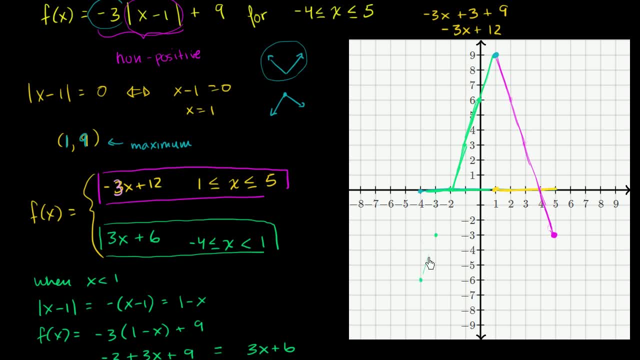 Decrease x by 1, decrease y by 3.. So it would look like this, It would look like that, And we are done. We have graphed this absolute value equation. Now, the whole reason why I did this is so that we learn it a little bit deeper. 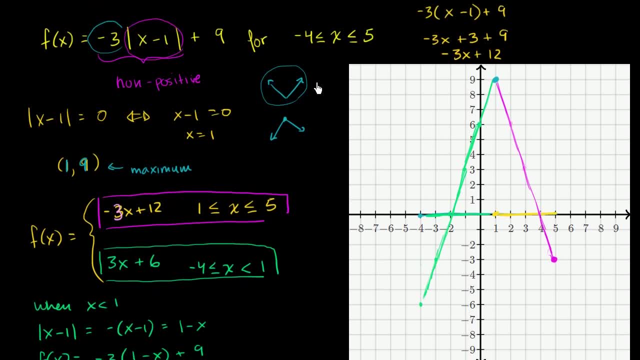 But there would have been a faster way of doing this. You could have just said: hey, this is going to hit a maximum point when x is equal to 1, because this non-positive thing is going to hit 0. So you could have said: 1 comma 9 is the vertex. 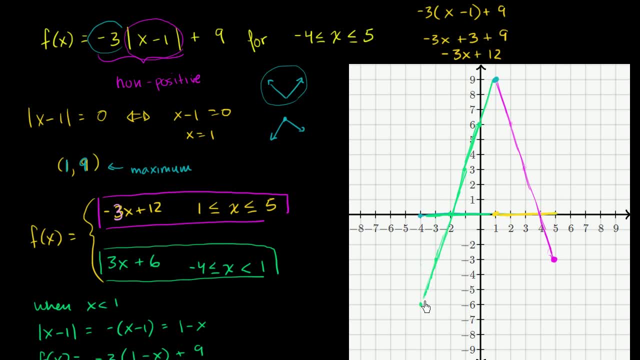 And then you could have just tried out the two endpoints, knowing that between the endpoints and the vertex you're essentially just dealing with the lines. You could have just evaluated f of negative 4. And f of 5, you could have figured out these endpoints. 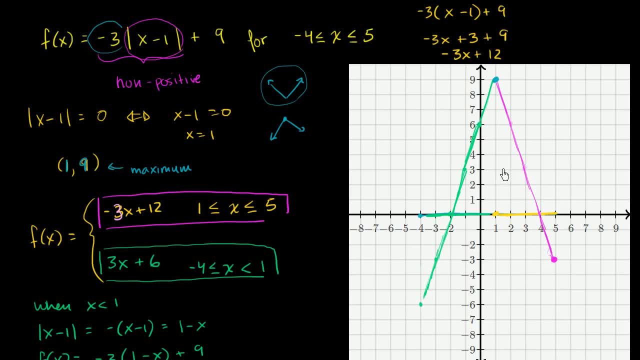 and f of 5, you could have figured out these endpoints and drawn the lines, But now we understand it deeper and that's always a little bit more exciting.